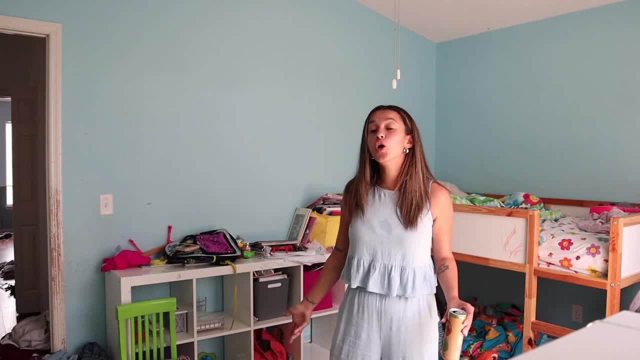 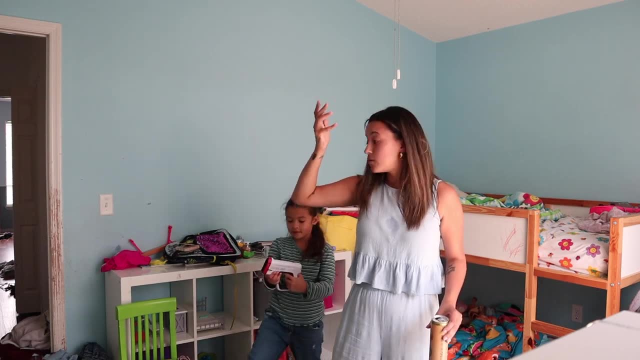 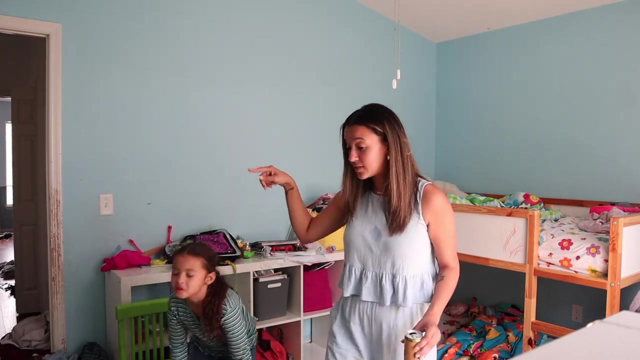 Because we like to wrap things Exactly. There's no excuse, None. Let me show you what we're starting with. As you hear, Stop, I'm cleaning. You are either going to help me clean up or you're going to go downstairs. Go get me two trash bags, please. now Let's go When you're at the door. 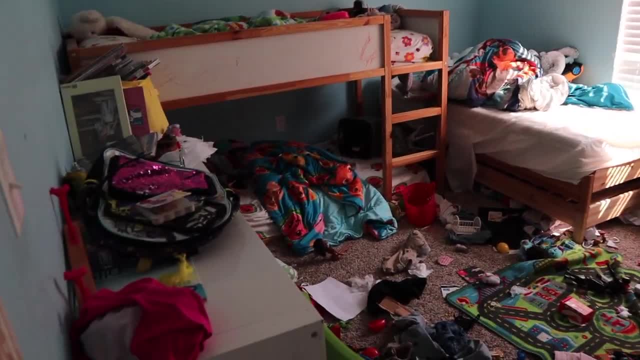 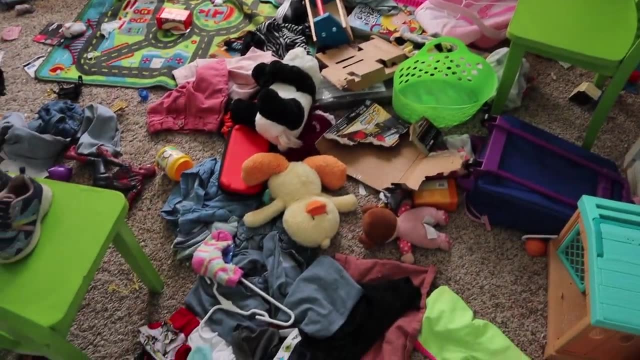 this is what you see. It is absolutely disgusting. My son's bed, This is horrible, Horrible. You're probably thinking: how the hell did you allow your kids' room to get like this? I just didn't have the motivation. 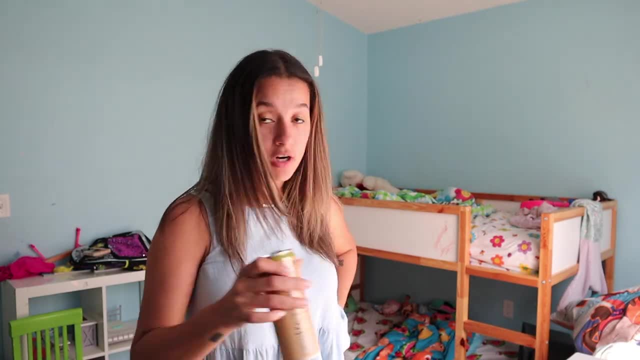 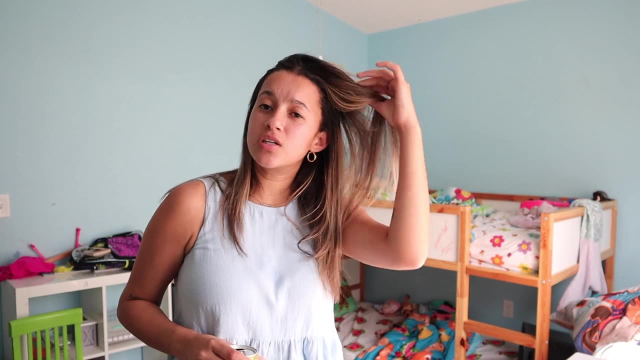 I would get off of work, I would come home, We would have our activities. We're going to go to the gym, They're going to play, We would have sports or whatever it is. By the time we got home and dinner was cooked and they're ready for bed, and I would see this. 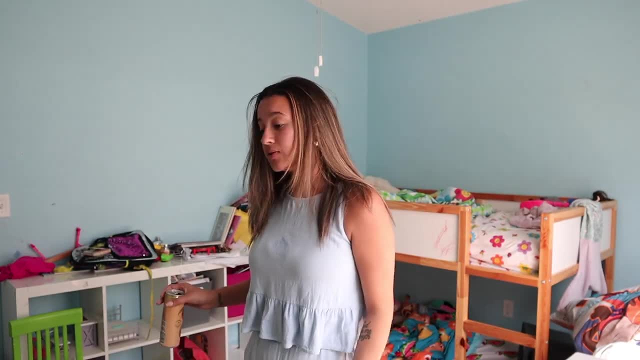 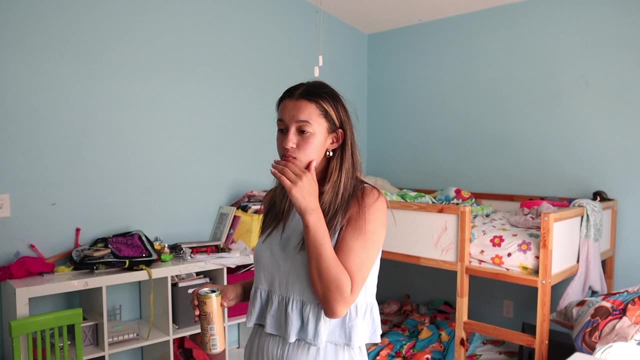 and I would tell them to come in here and clean it up, And this is still the state that it is. Ultimately, I think it's just too much stuff for them. I think we need to go through a lot of stuff, get rid of a lot of stuff and make it more minimal for the things that they actually play. 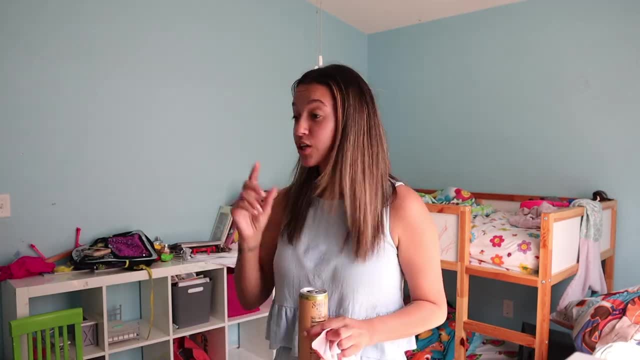 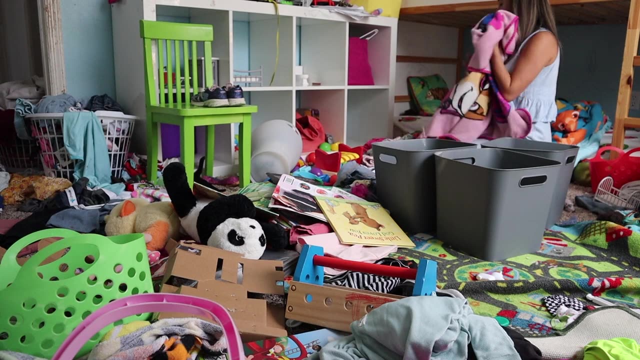 with and use. I'm just overwhelmed. I got me a beverage, I'm going to throw on some music and we're going to get to cleaning. I ran away from heartbreak. Got nothing in return. Got nothing in return for my pain. 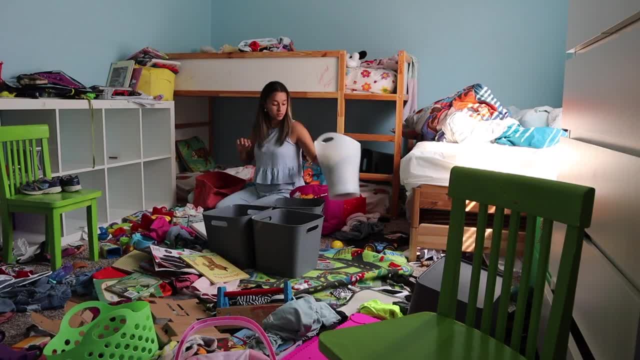 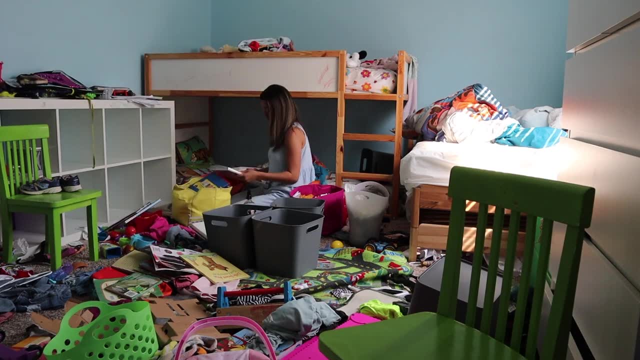 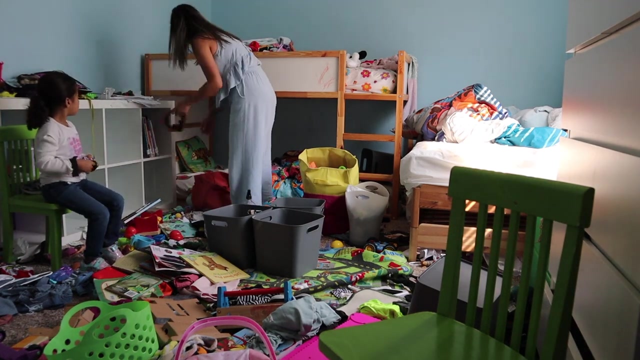 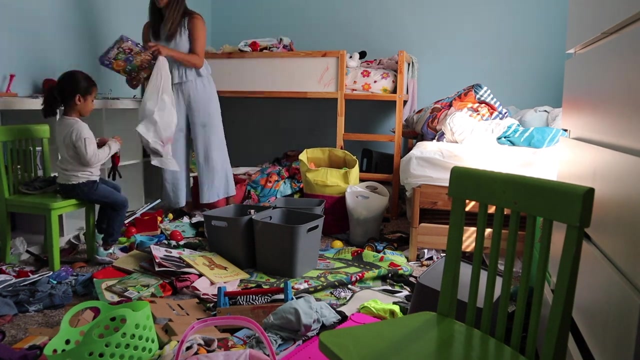 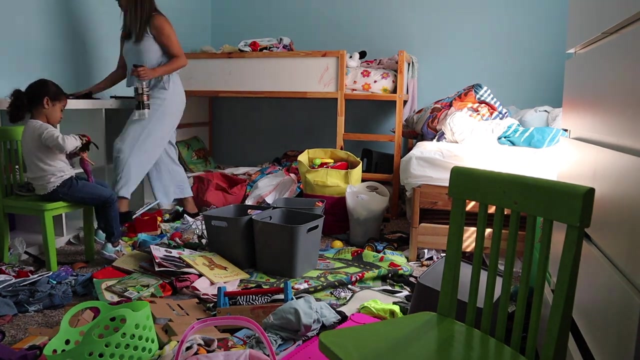 I never thought I'd be so empty, so alone and afraid, Wasn't looking for a lover. Nobody understood where I've been. I guess I thought I needed more time to protect my not from potential offense, So I held it in. then you came around and you made it go, but I shut it down. 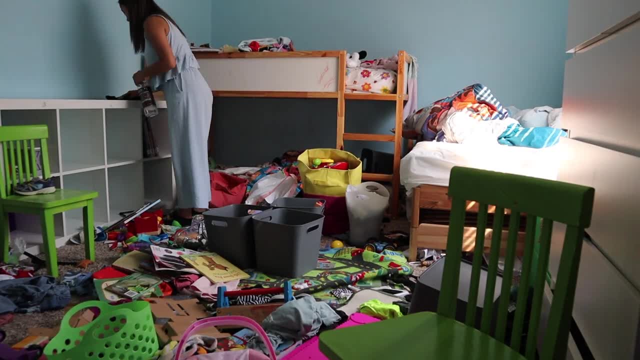 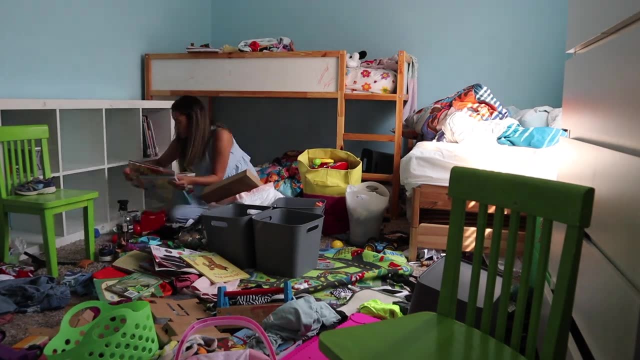 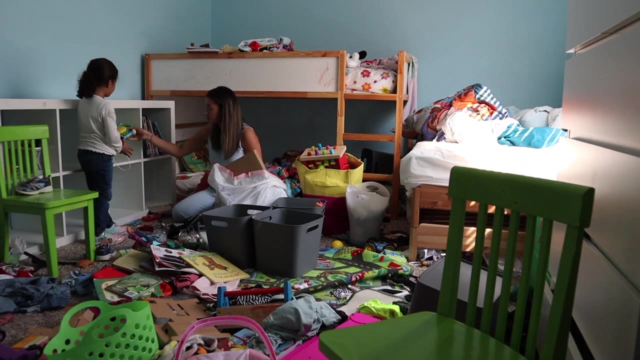 So you took it to heart and I opened up. I'm not surprised by what I found, cause I know I needed something different and you had to know I want to see it, cuz I know it had to be you, Out of the blue, somebody who listened, and it had to be you. 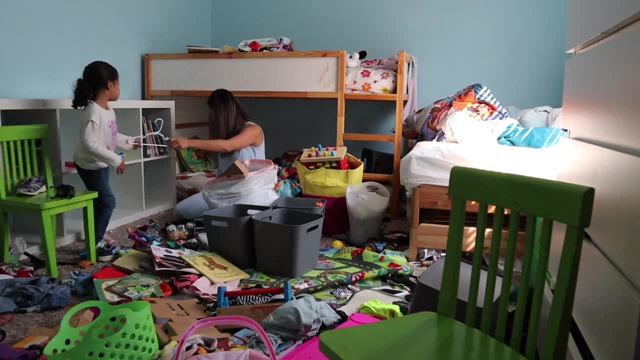 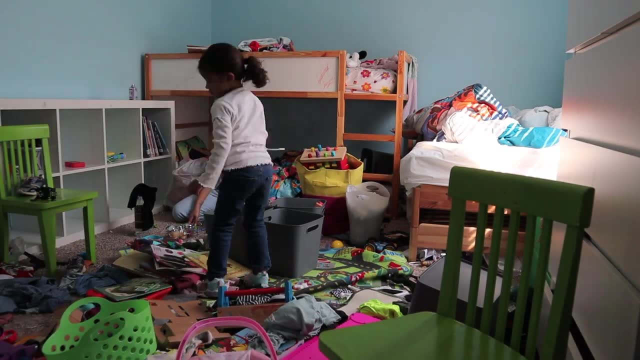 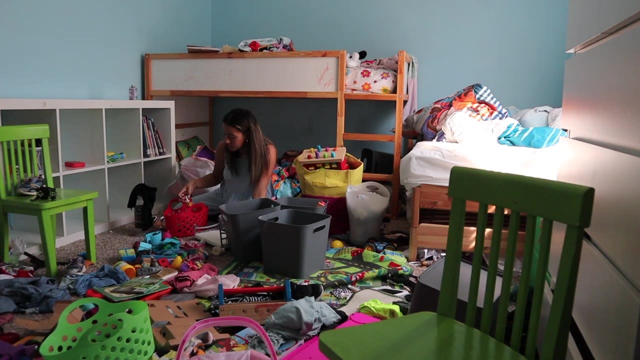 Out of all the people to reply, my love couldn't be just anyone. It had to be you, My baby, it had to be you. It had to be you. I didn't seem to notice, but you were checking for me. 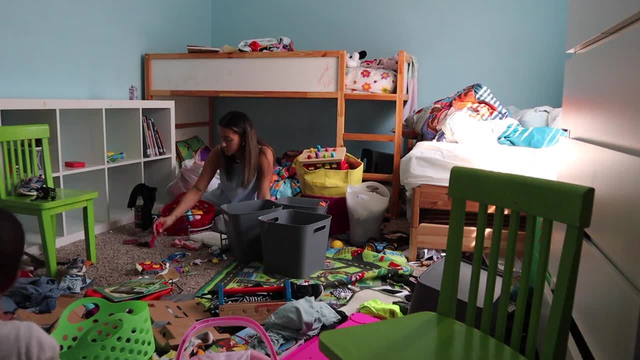 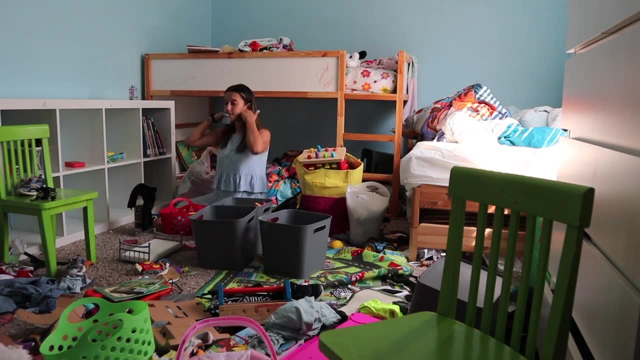 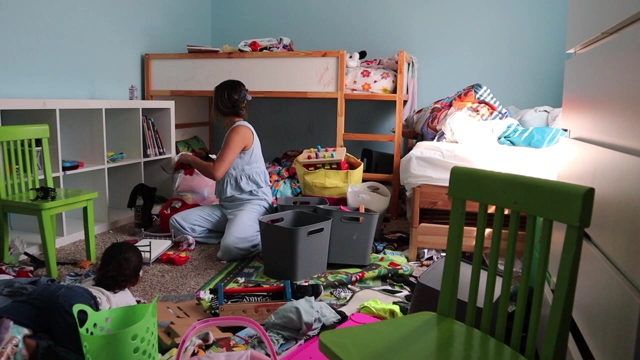 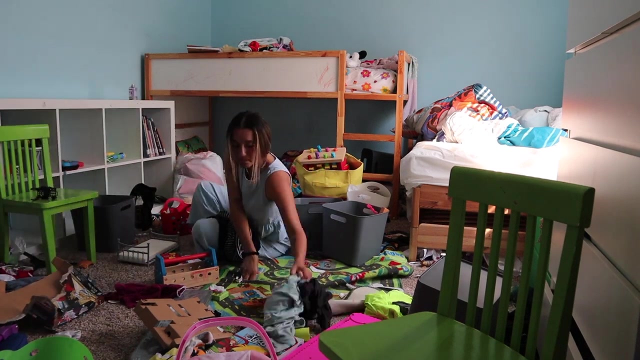 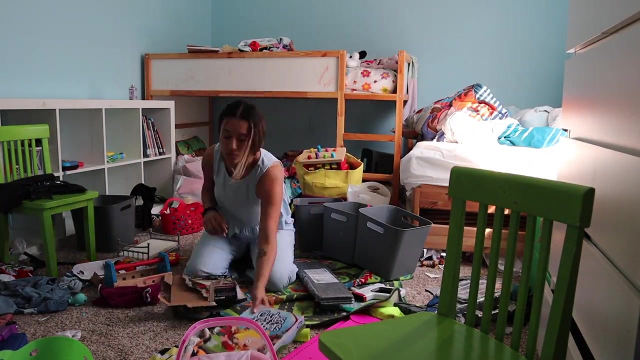 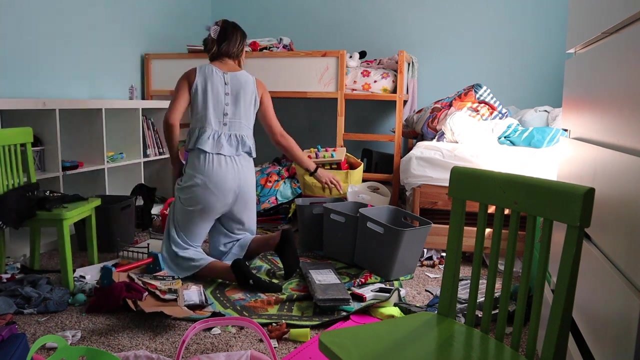 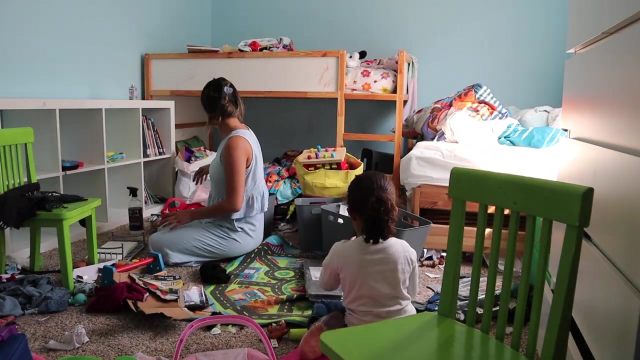 So we started building trust and my fragile heart started to bend. I should have paid attention. You would have been the obvious choice, But I needed time to see, clearly, Dig deep and cut through the noise. So I, Then you And you, But I, So you And I Opened up. 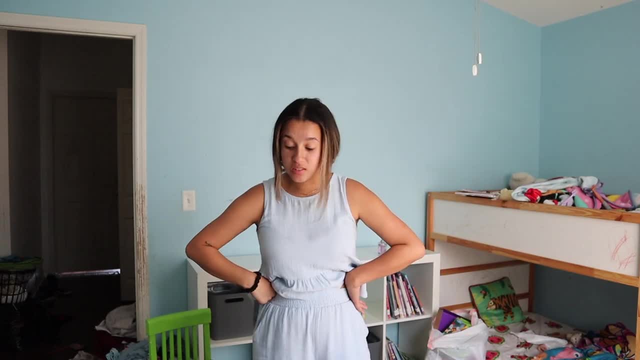 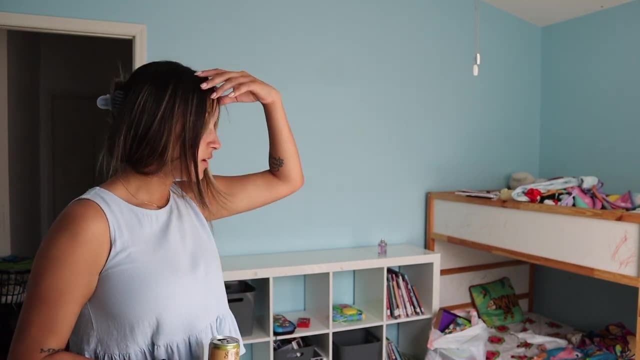 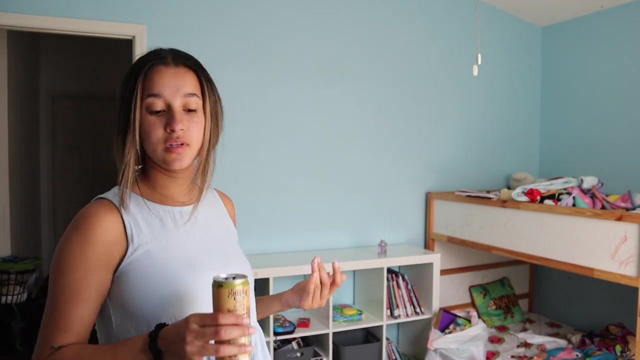 The room gets so hot when the sun starts coming out, I've almost Um Filled up an entire trash bag. Um, Yep, I just don't understand my kids, Like I really don't. So I've made a little dent on the floor right there. I've cleared off this. 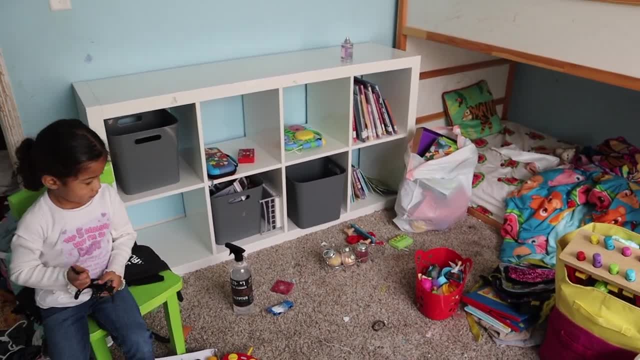 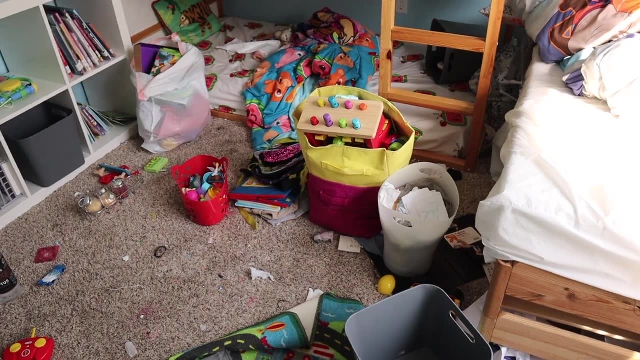 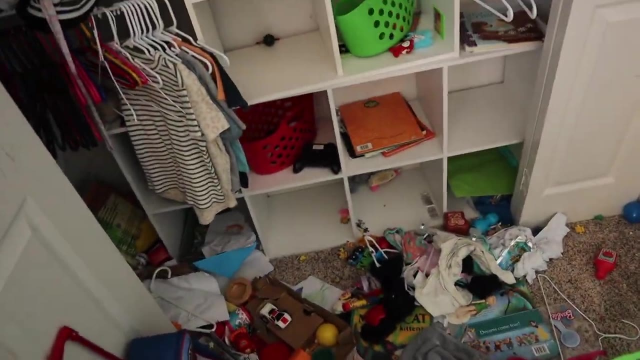 Trying to make The best use of it. There's my trash bag almost full. I have another one on one of their beds, And then that stuff is pretty much either donation Or trash. Um, And now we have Like clothes over there, Just more random stuff, And then we have to tackle this. 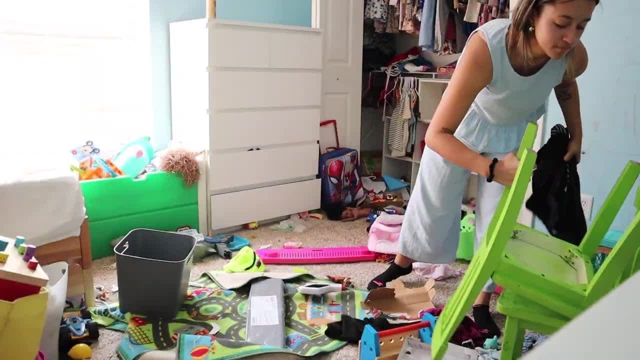 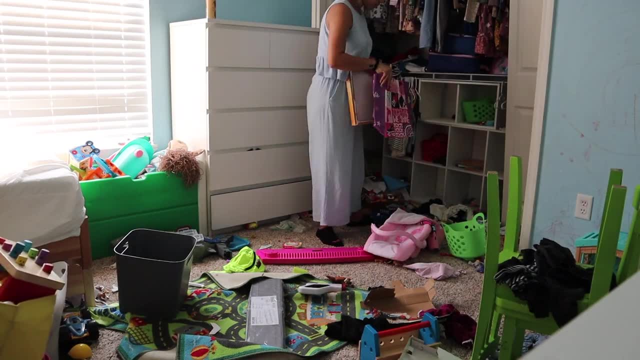 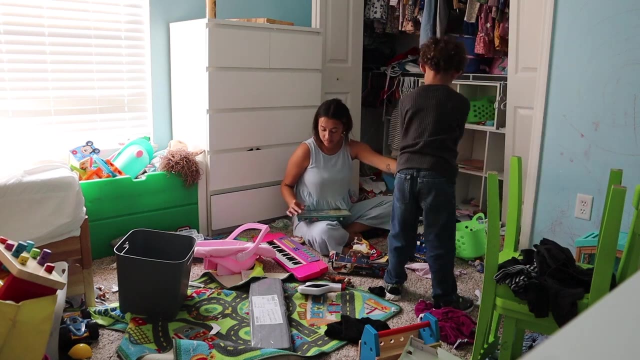 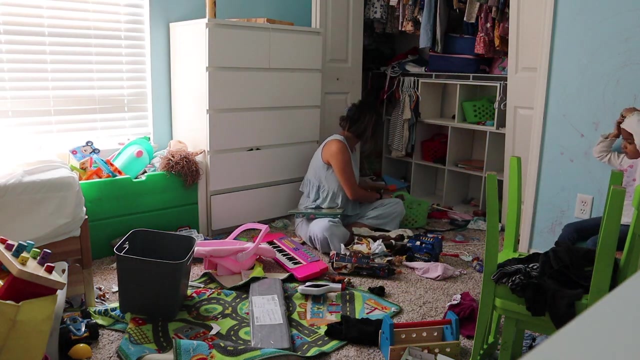 I also need to make all of their beds. I also need to make all of their beds. Living for weekends, Wishing I could take a break from this world Running on a hamster wheel. But searching for something I can't find. But searching for something I can't find. 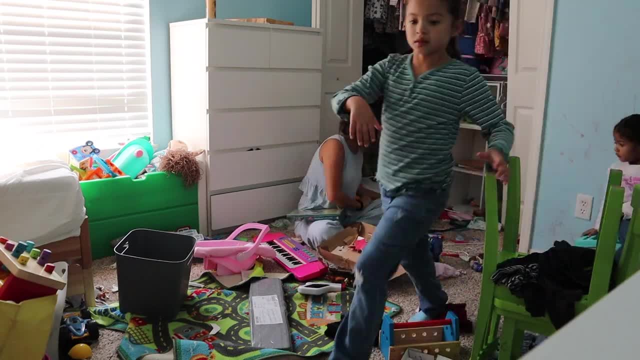 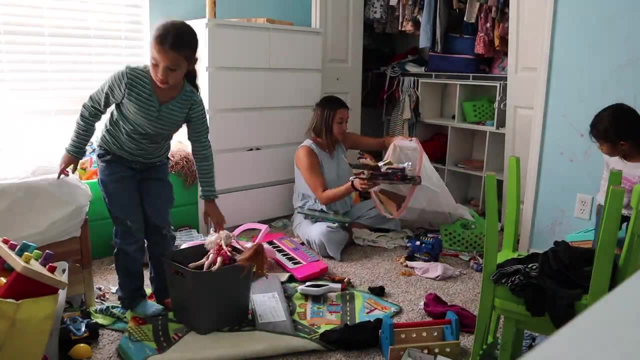 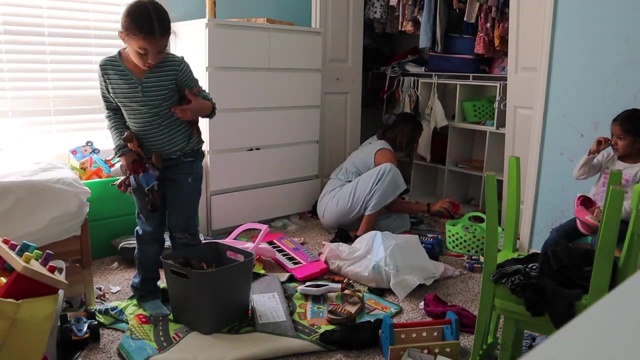 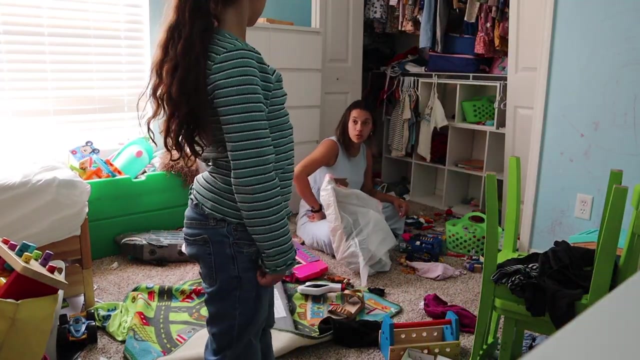 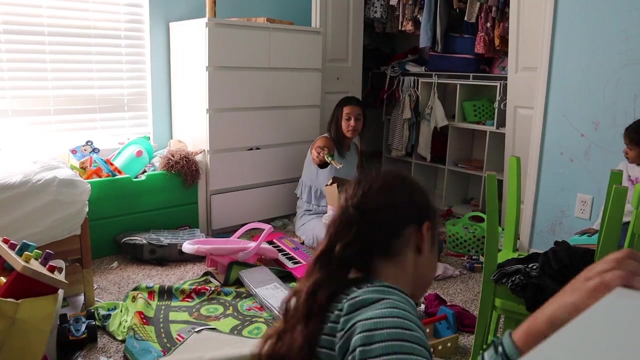 I just wanna Be a lost girl And fight, Take a breath, Feel my wings spread, Levitate above the ground And make eye contact with clouds. Now I'm rising, I'm soaring Above it At all. I just wanna be free, Finally, Finally, Finally, Finally. I wanna be free. 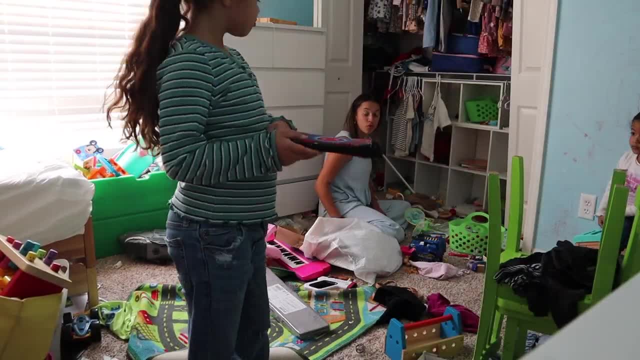 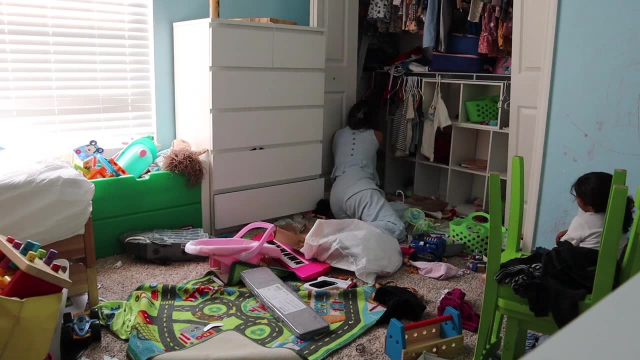 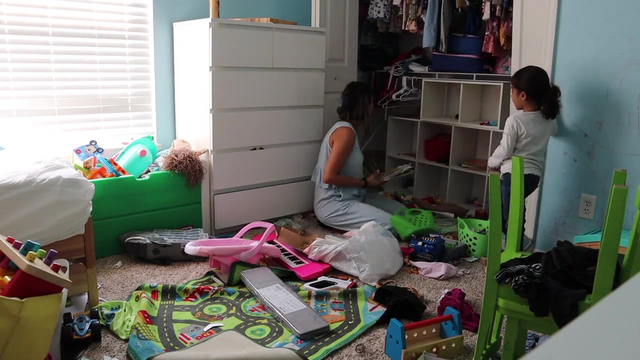 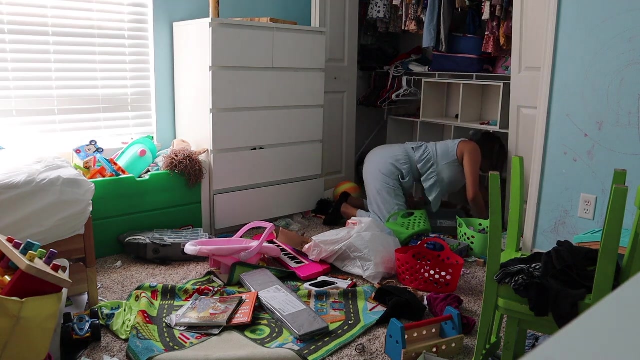 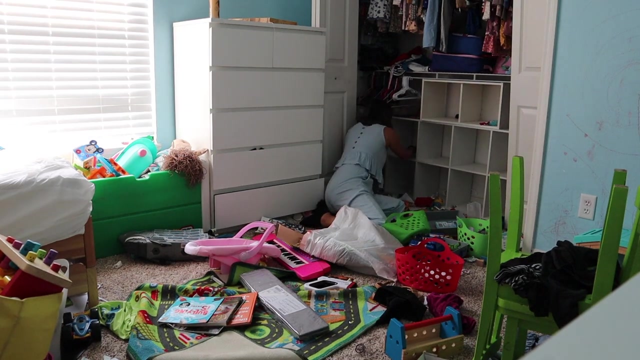 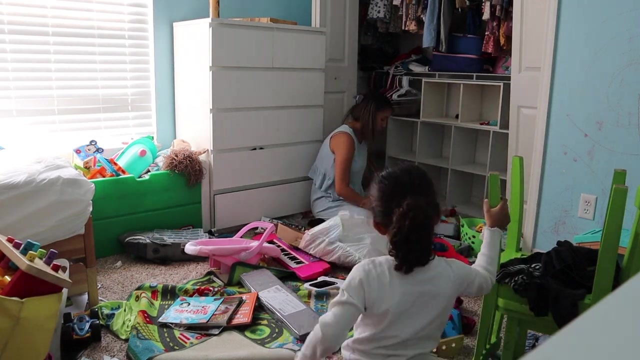 I wanna be free. I wanna be free. I always stay dreaming. Never imagined I'd lose my spark, Living in this crazy time, Putting back the pieces of my mind. I know how to run from the dark And fly. Take a breath, feel my wings spread, Levitate into the clouds. 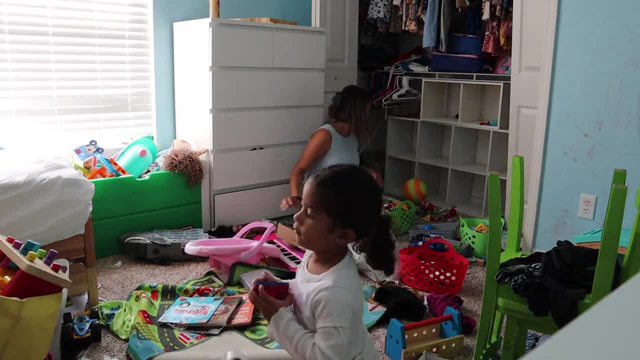 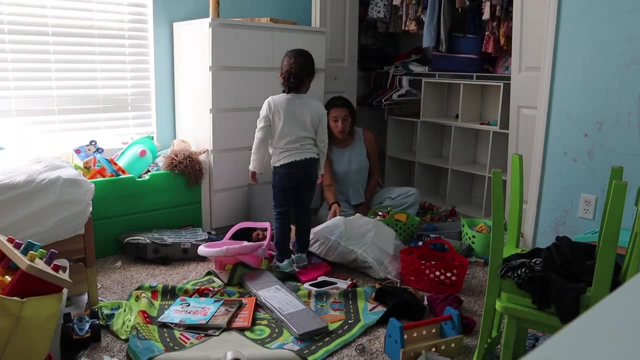 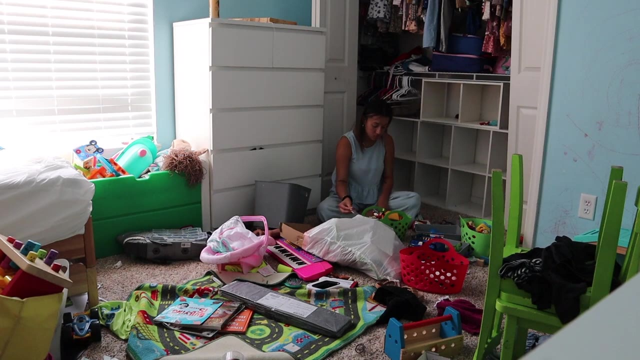 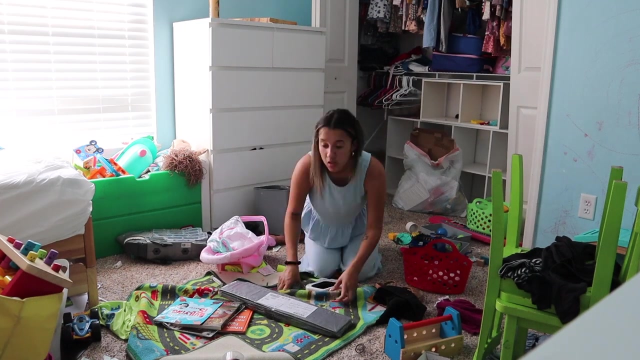 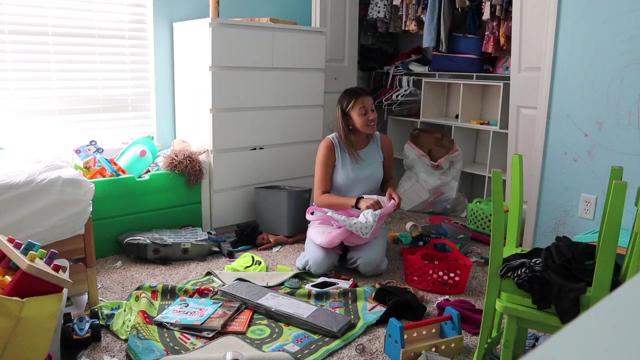 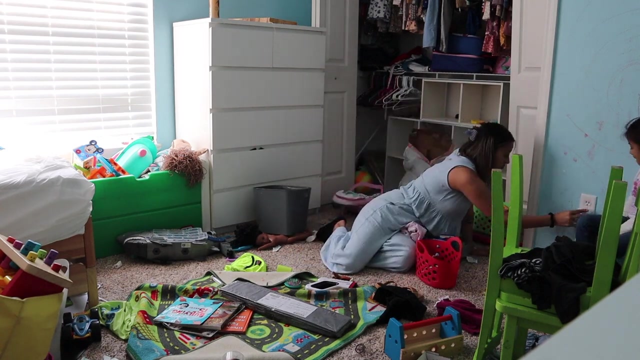 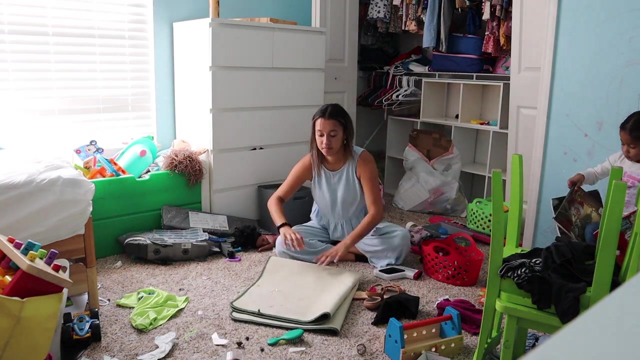 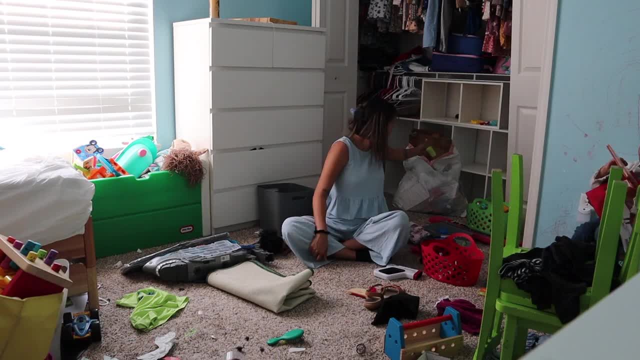 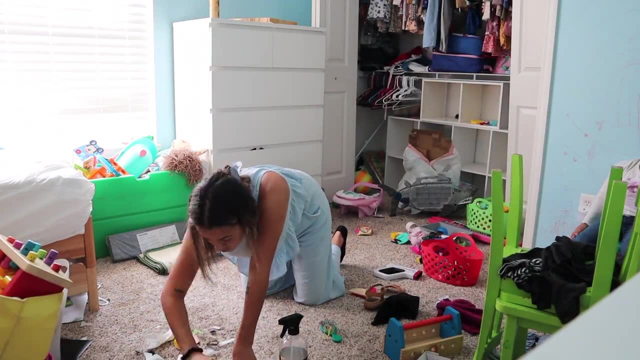 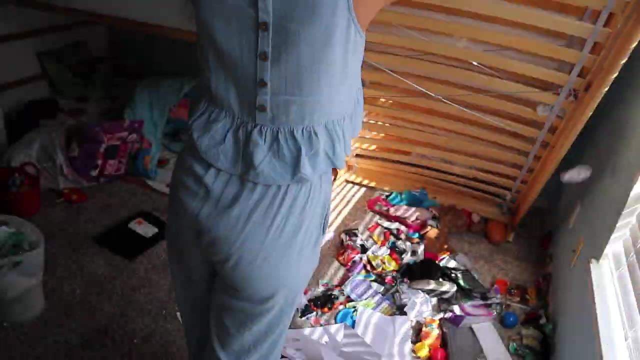 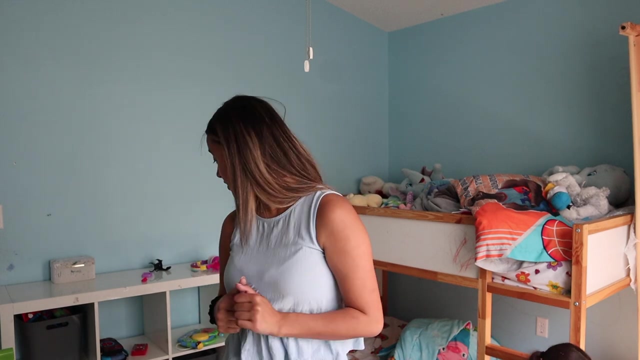 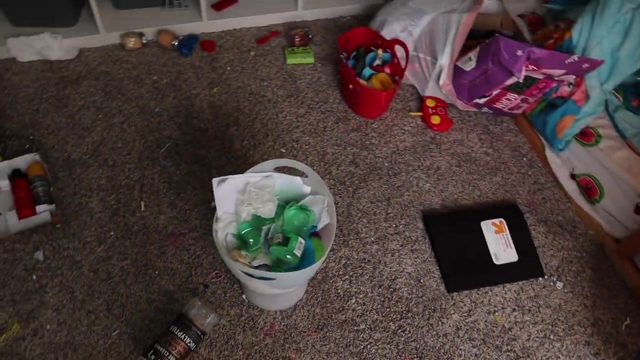 I just wanna be free. I wanna be free, I wanna be free. I feel like I'm making progress. It's just never ending Like I just lifted up my son's bed And all of this was underneath his bed. We are making progress with seeing the floor, Whoa. 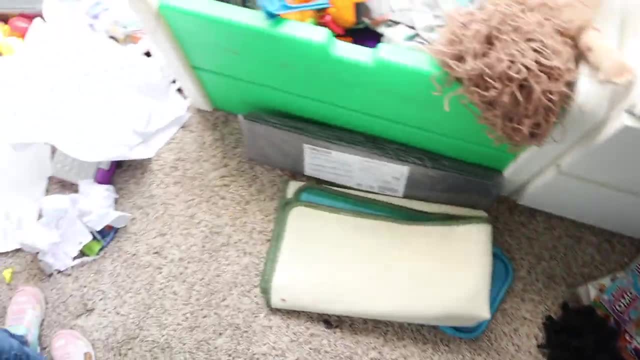 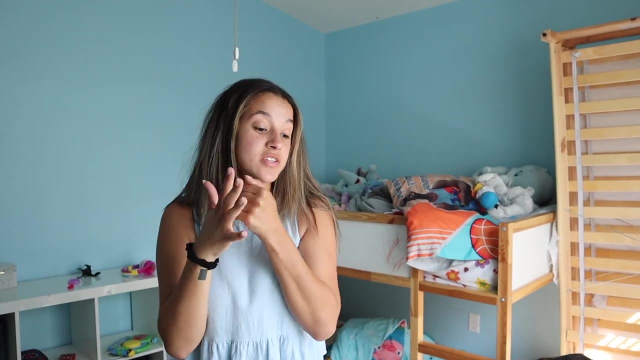 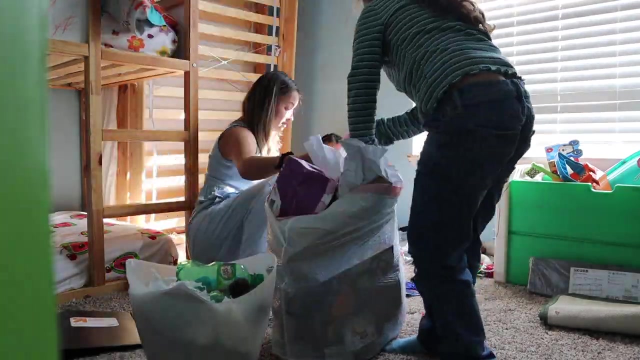 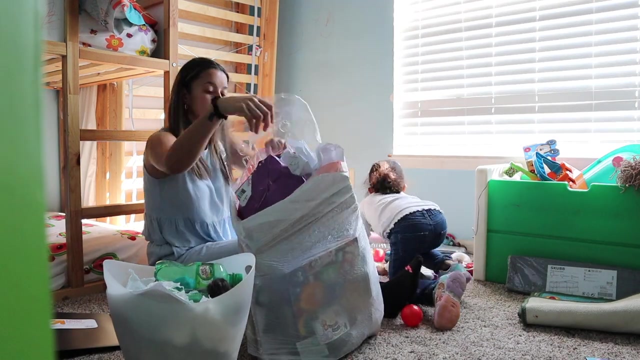 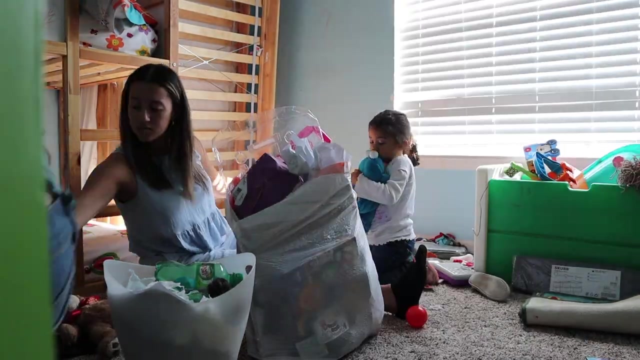 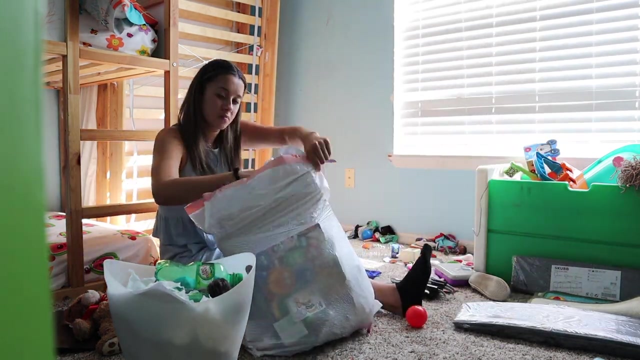 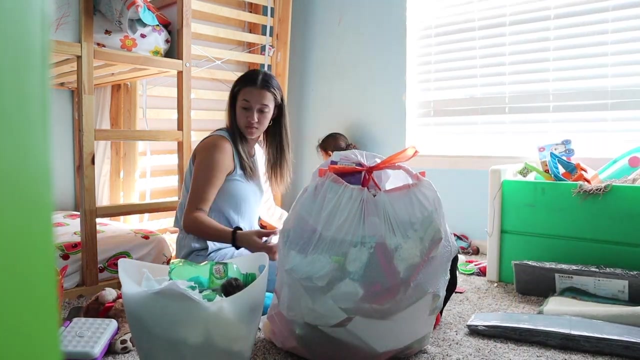 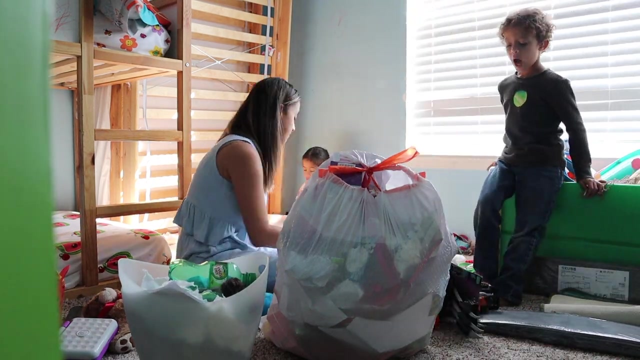 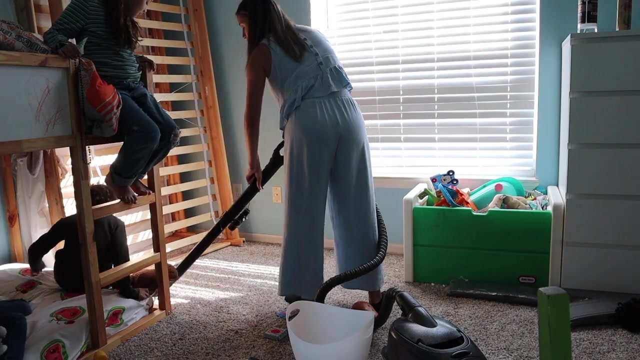 There it is. And why is stuff sticking on the wall? I just, I'm just, I'm overwhelmed. I just don't understand why it's this bad. Don't see the ends of his head? Oh no, It's the next day. I got very overwhelmed First. my battery died. 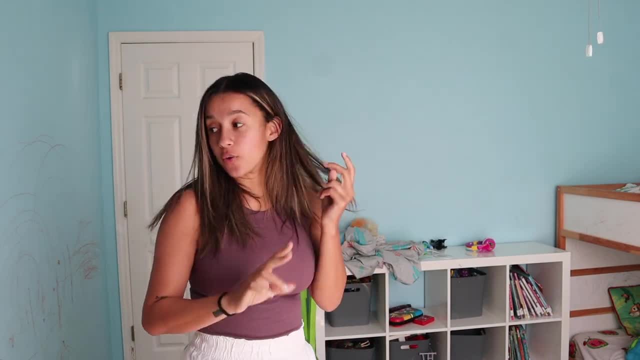 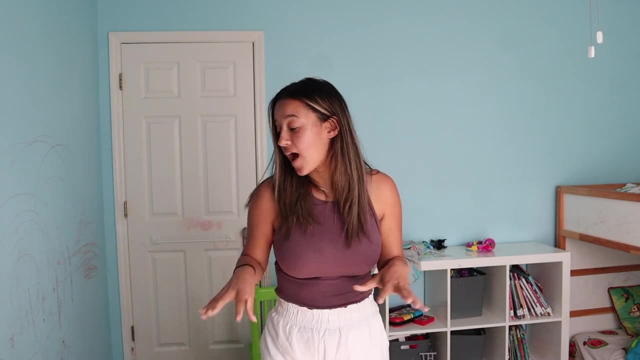 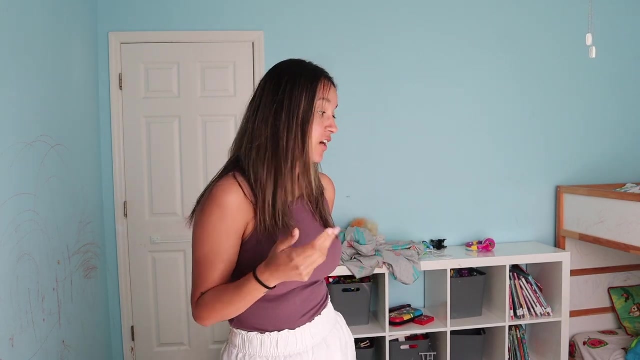 So I couldn't finish recording yesterday And I just got overwhelmed. It really bothers me with how chaotic my children's room is. We're changing it Like I cannot have it looking like this again. It's embarrassing for me And it's not good living conditions for them to have all this stuff. 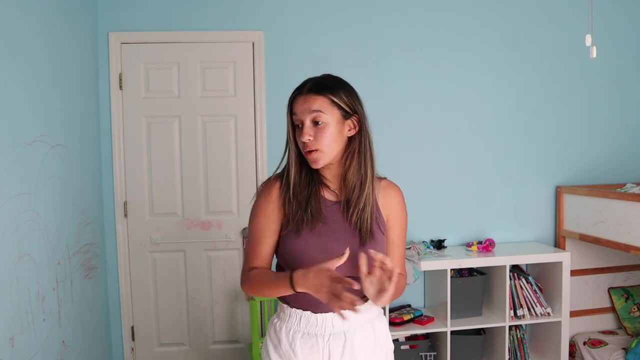 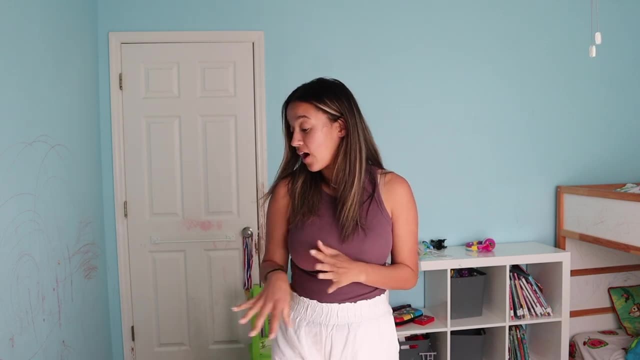 So we've made progress. I will show you what I'm working with. I don't remember what time it is right now, But we have taken a lot of stuff out of the room. I threw away two trash bags full of crap, And then I have two trash bags full of crap. 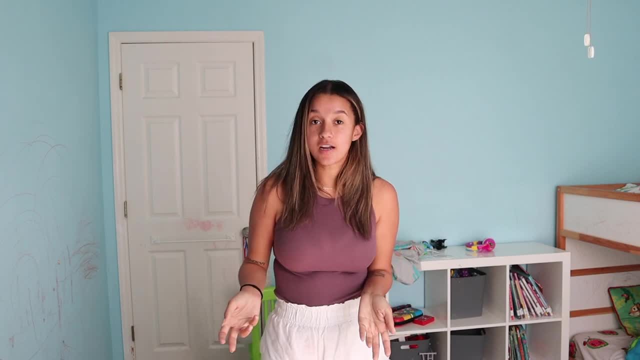 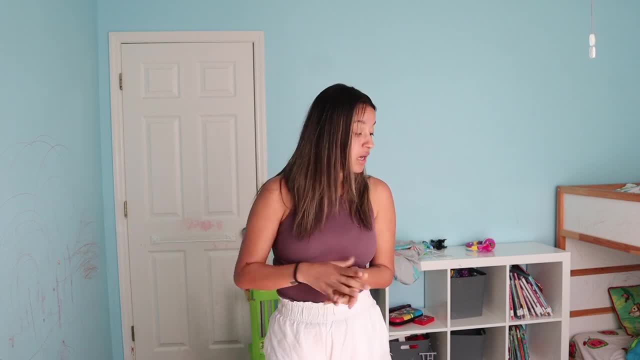 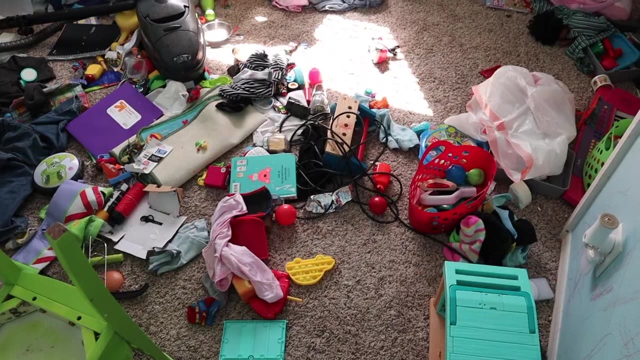 So I'm taking all of it to Goodwill And I'm only keeping what they actually use and play with. So let me show you where we're at now I'm standing at the door again And it probably doesn't look that much better. I mean, we've made progress. 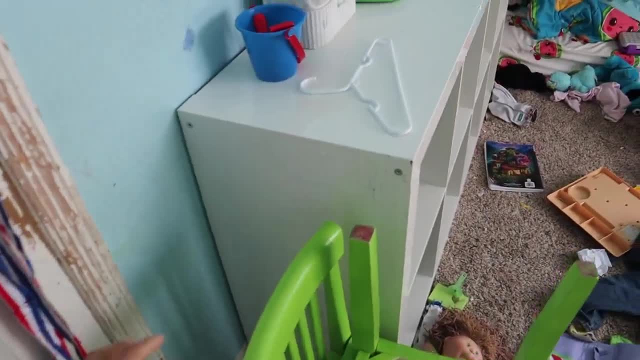 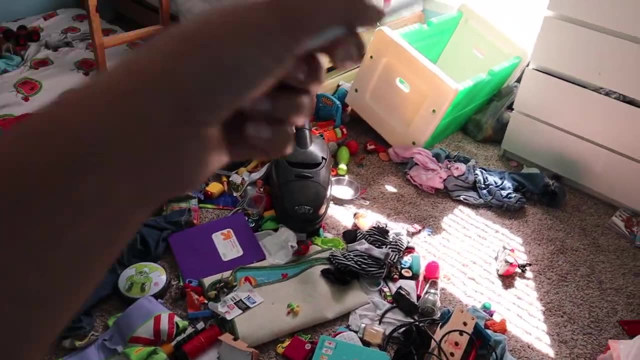 This is dirty. I need to wash all the kids bed sheets, But this is what we're starting with this morning. Honestly, it's not that bad. What made it worse was I dumped out that. I think I did it after my camera died, So everything that was in there is now on the floor. 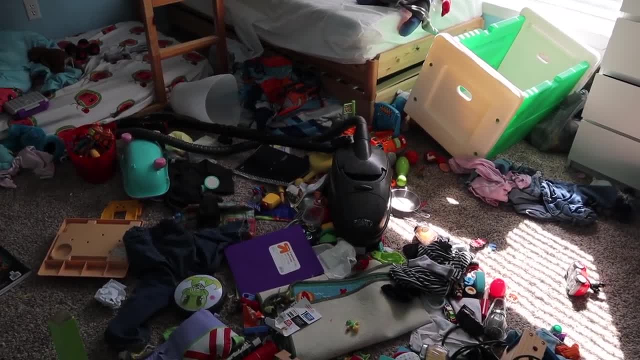 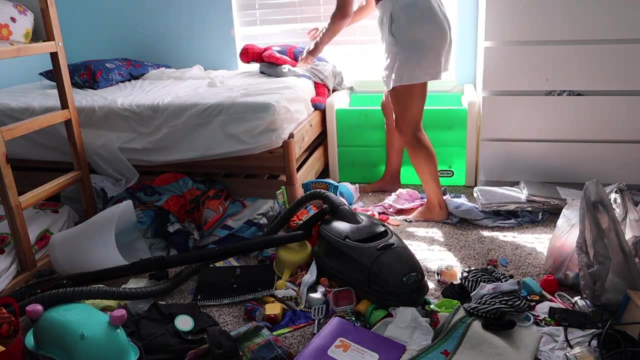 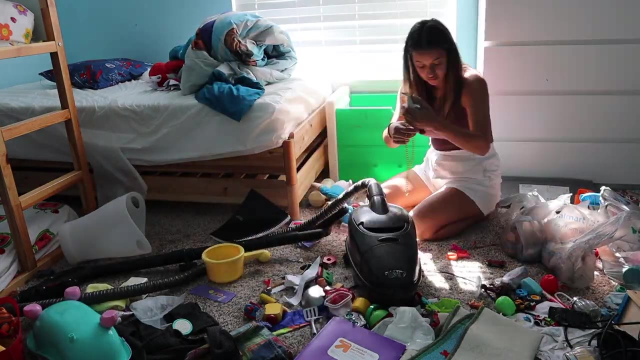 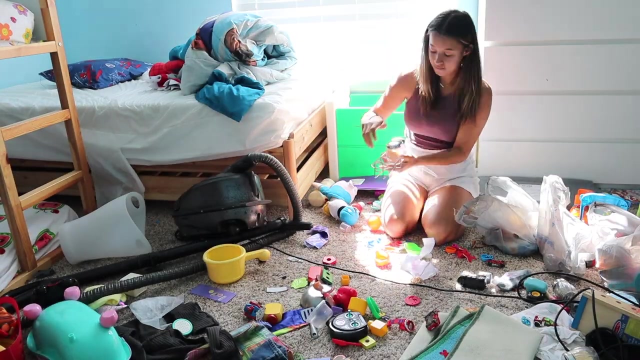 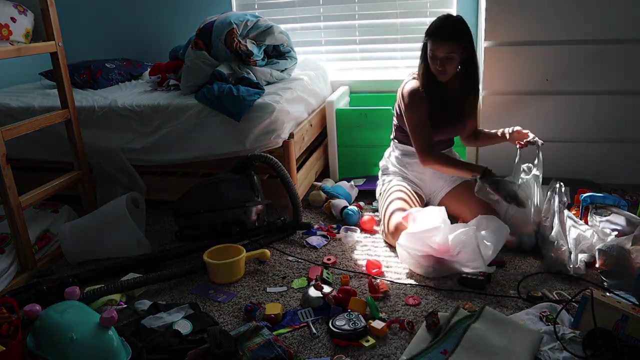 So that's why I'm like, oh, it's not that bad Because we have made progress, But this is what we're starting with this morning. This is not how I wanted it to be. I totally owned Oh, and I did what have to be done. I really can't get over trying to figure out I can fix my wall. 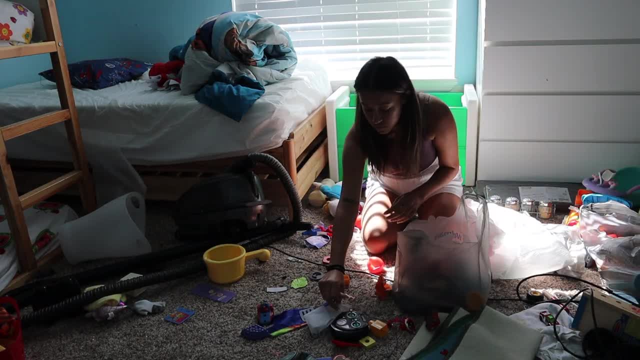 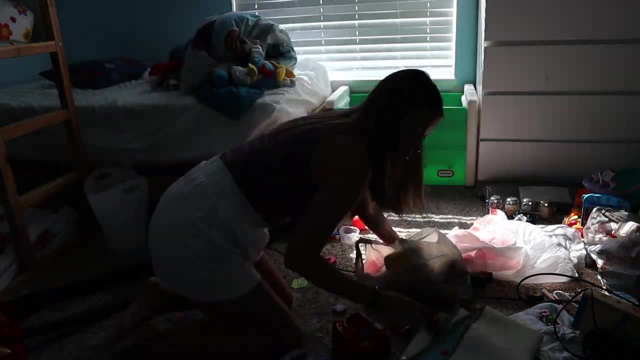 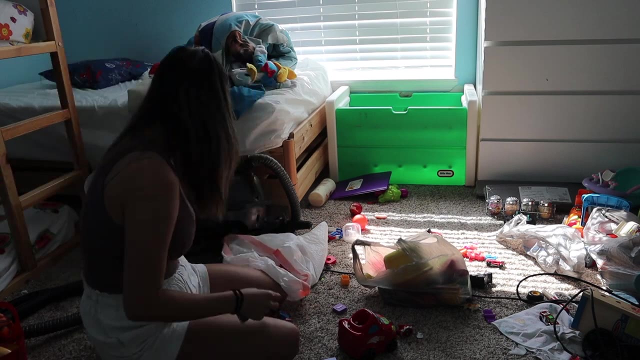 I bet that happens dancing, And sometimes I fell off. That's because of what I did. I mean, God saved me, But I could've done worse. This house needs construction. This house needs construction. It just won't make anything. This house needs construction. Maybe if the grid is a adjuster. 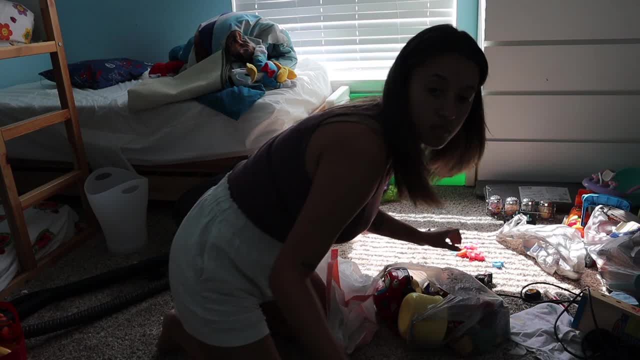 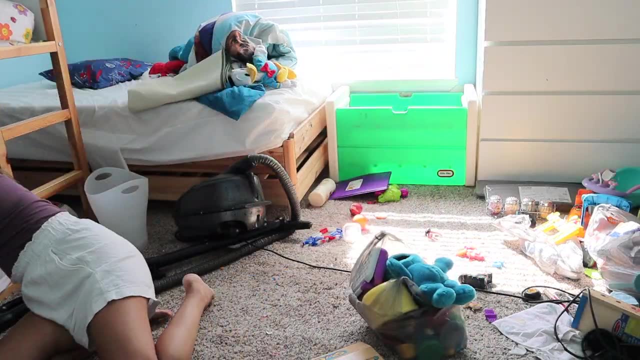 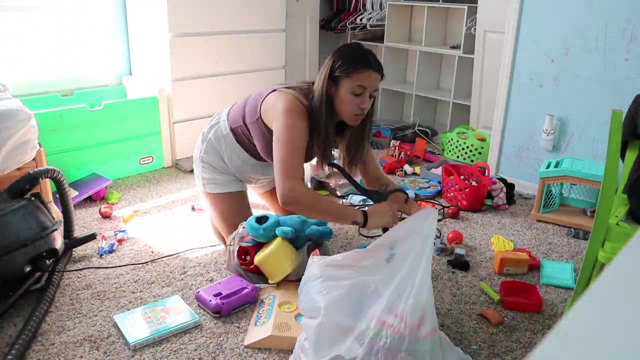 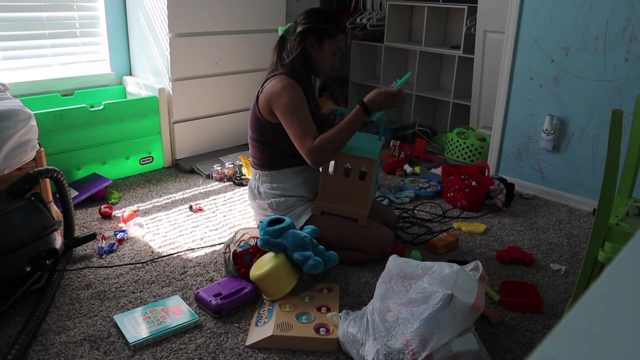 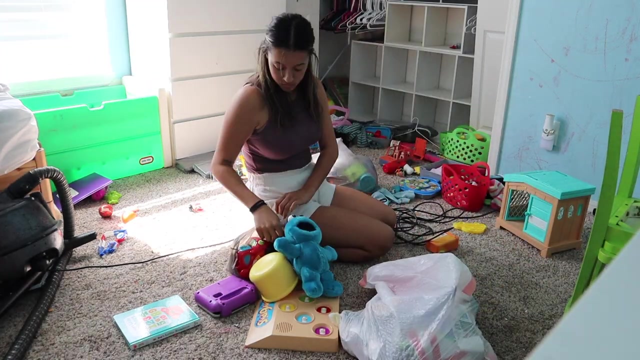 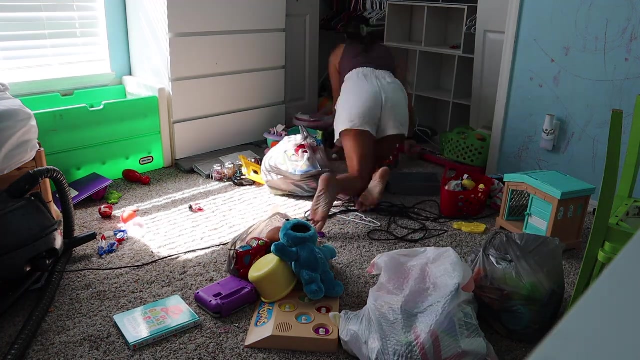 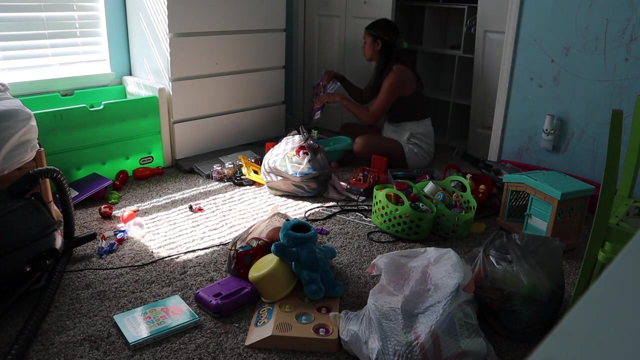 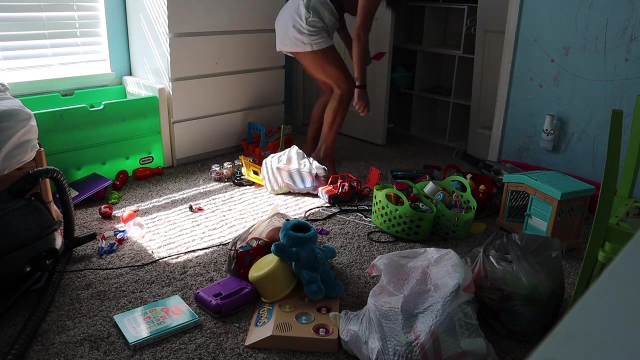 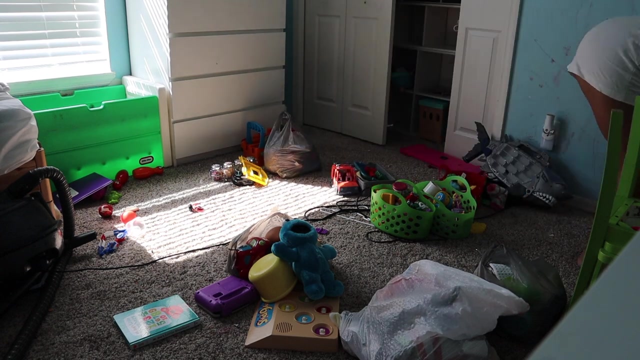 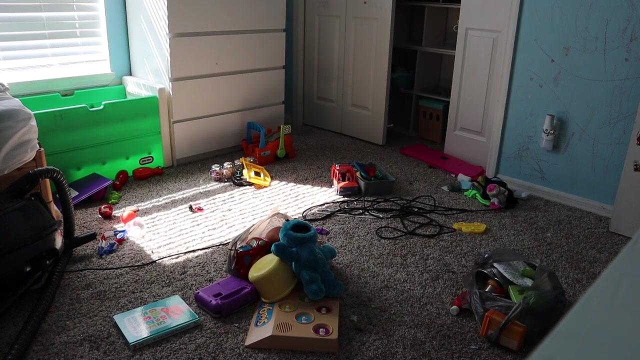 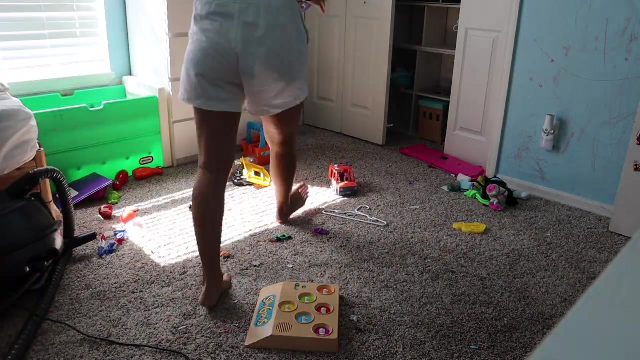 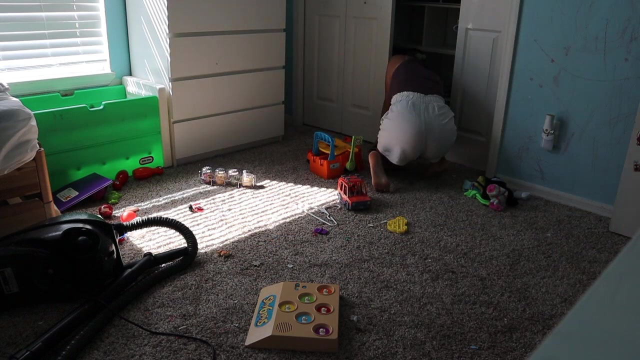 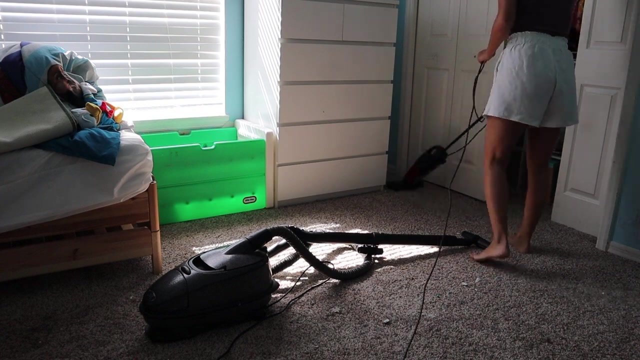 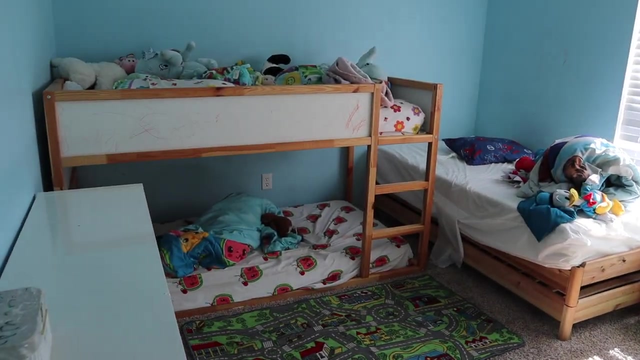 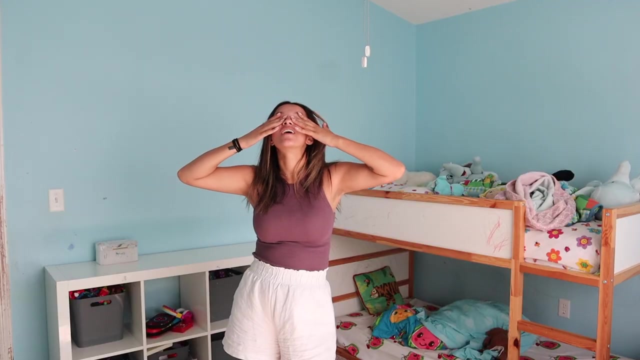 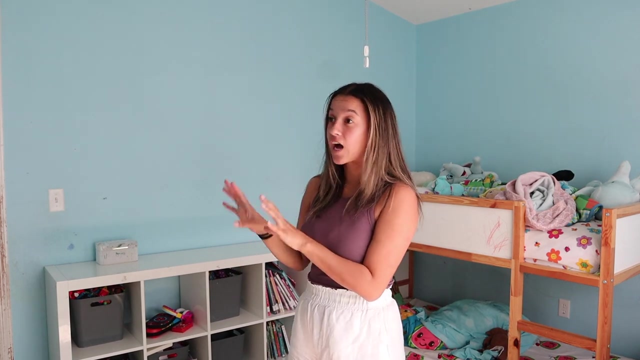 Maybe if the grid is a adjuster. Thank you, Thank you, Thank you. It is finally clean. I just have to clean the kids' bedding, which I'm going to go do now, but I have four trash bags of trash outside their door. 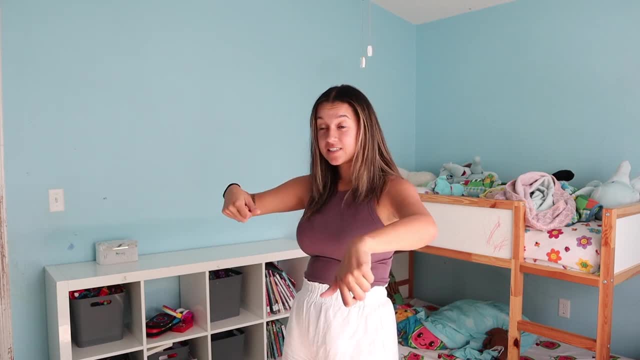 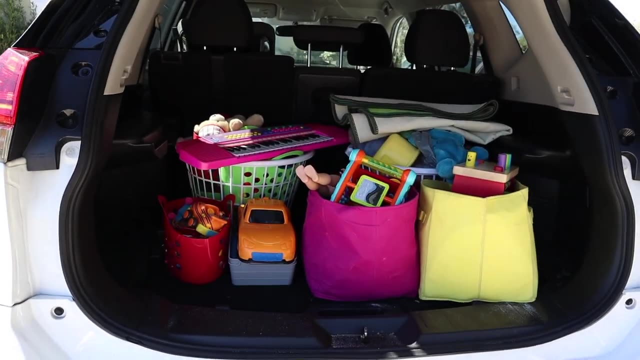 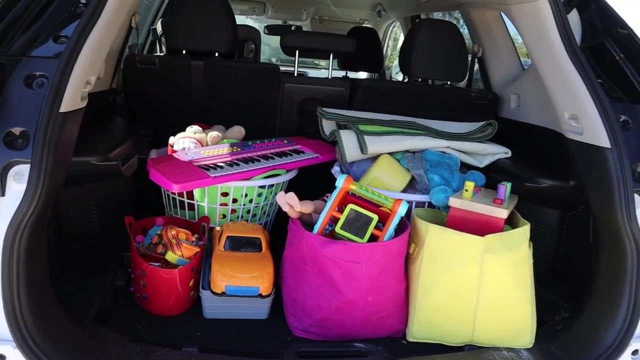 And then I have two laundries, Three baskets full of donations, And then I have like a keyboard that they don't use, And then they have two card track rugs. I'm getting rid of one of them, So I'm going to move all of that into my trunk to take to Goodwill. 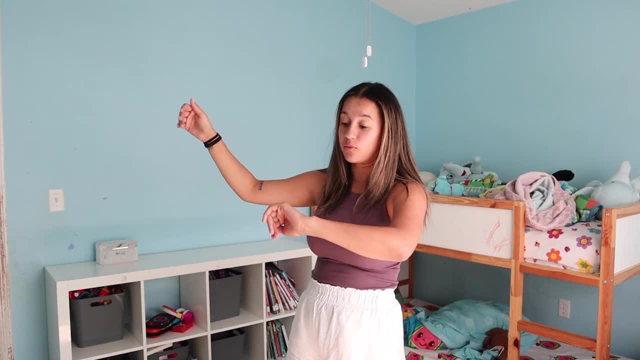 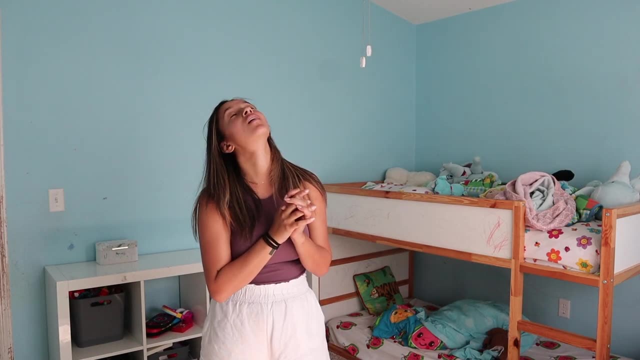 And then one back. when I clear out the hallway, which we'll do now, before we leave to go get them from school, I will throw their bedding in the wash so they'll have clean sheets, clean room. I'm praying it doesn't get chaotic like that again. 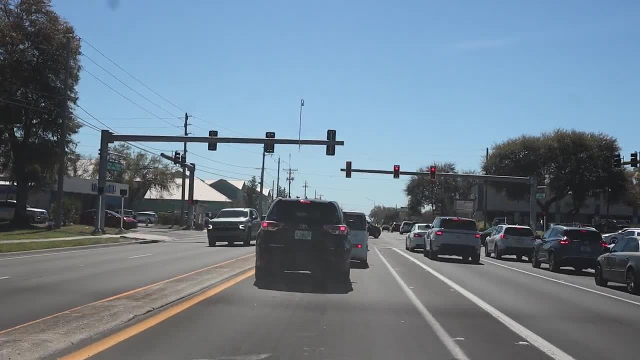 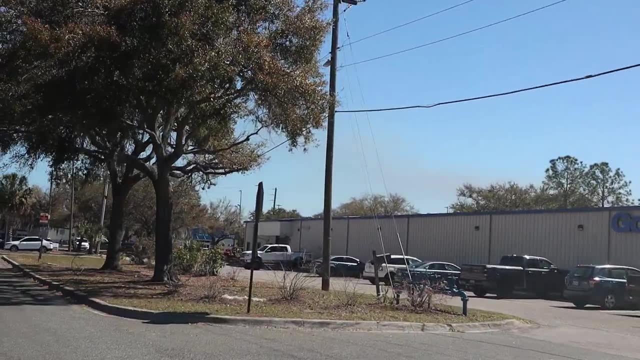 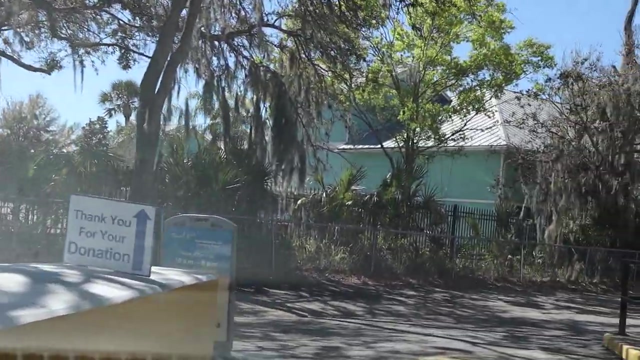 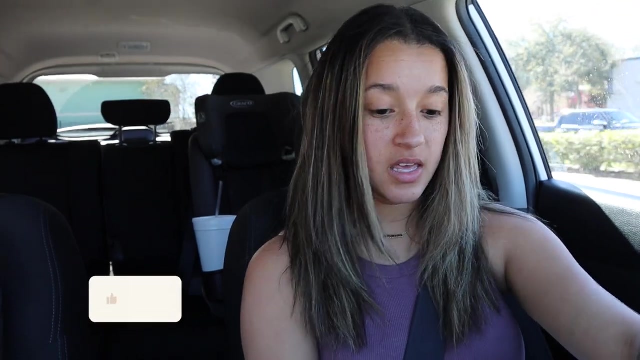 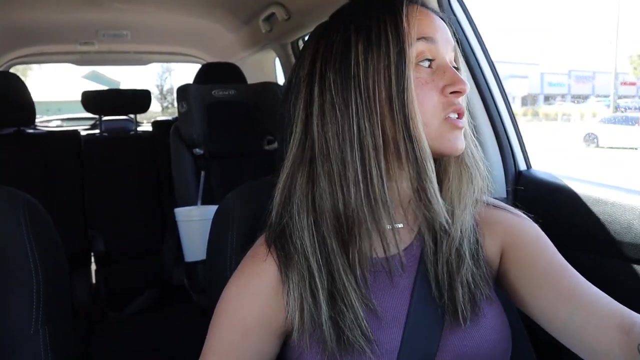 I feel so productive, I'm so proud of myself. That's something that I needed to do for a very long time, And just with work and everyday stress, I just haven't had the time, Especially Like yesterday when I was trying to clean and then my kids ran in and they're like 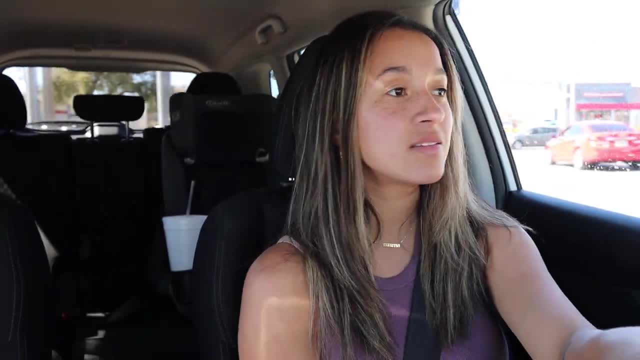 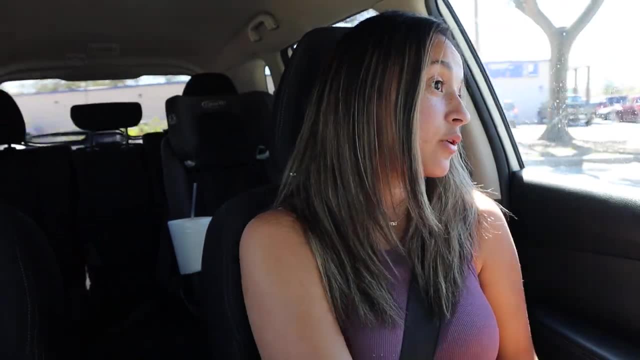 Oh no, but not this- A toy that they have not played with in months. All of a sudden it has so much importance to them And it just became overwhelming. So I just never had time to clean the room, because I'm always with my kids. 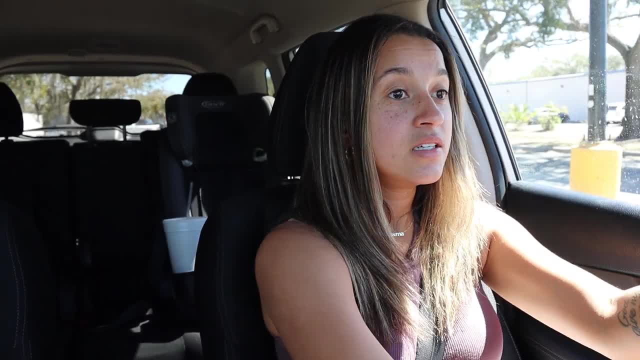 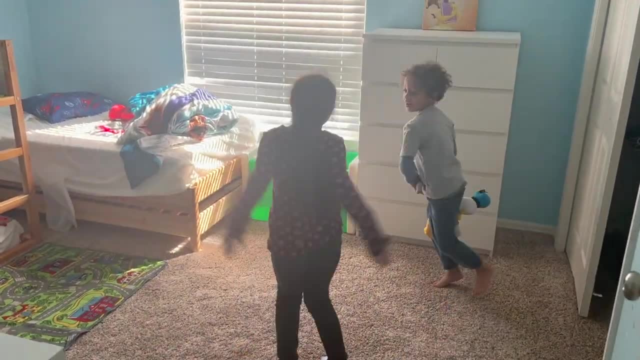 But I have this little bit of time, I'll turn here To get it done. Just oh, it feels so good. They're going to be really excited when they get home and have a clean room. What I still need to get done with their room. 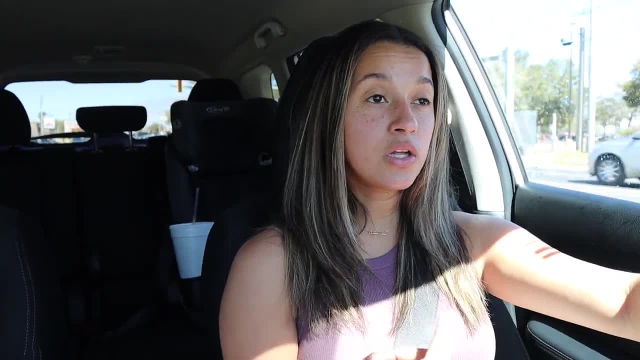 But I'm not. I'm not going to record. I need to go through their clothes. They have so many clothes, But like a lot Like my son recently went through a growth spurt, So like his long-sleeved shirt. 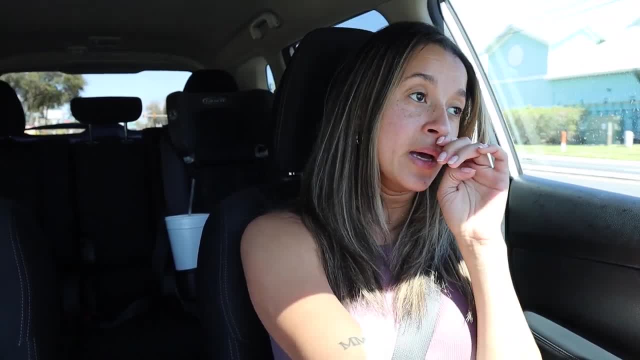 Some of them don't even fit him. They're like very short on him. So I need to just go through their clothes and try to sell what I can at Once Upon a Child And whatever I can't just take to donation as well. 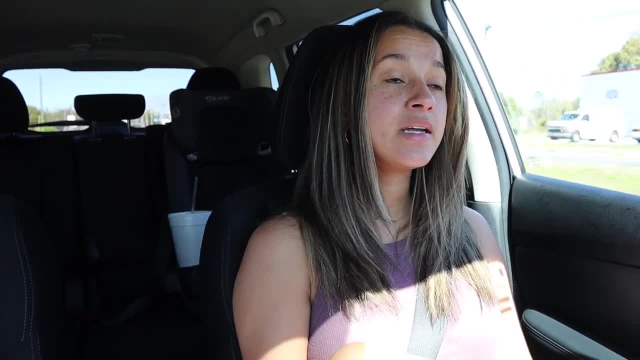 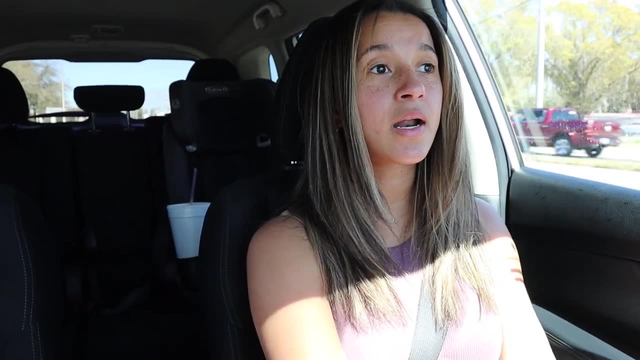 And then they have like a Lego table that I got. that I want to move into their room, So put that in there. My oldest daughter got a Barbie house for Christmas that hasn't been brought upstairs to her room, So move that. 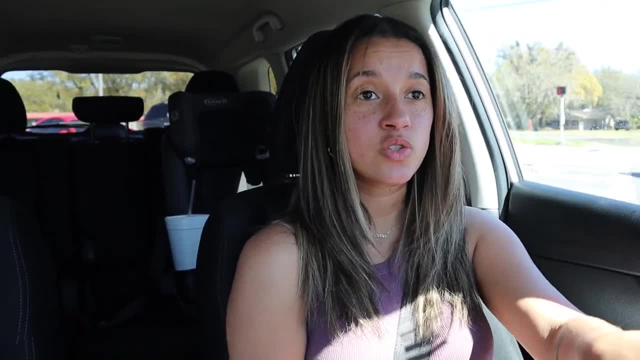 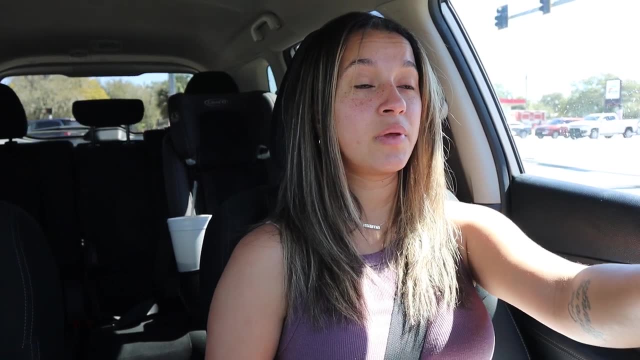 I'm going to put that up there, which I'll probably put where their toy box is. And then my son also has a racetrack, But it's really big And I don't know if it will fit in their room without being too cluttered. 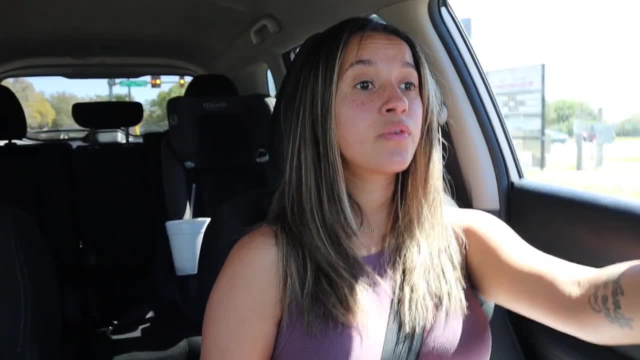 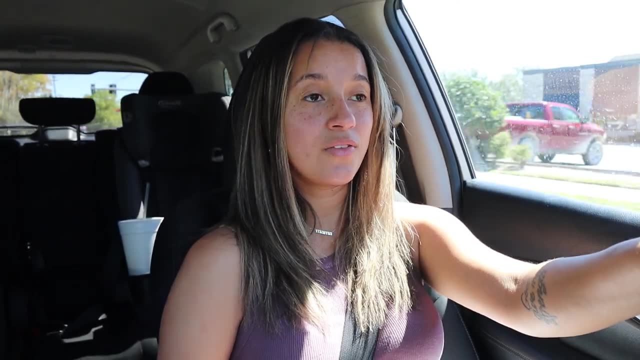 So we'll see, But I'm going to just put everything in their room that they actually play with, instead of having all these random knick-knack toys that they don't even know what to do. They just dump them out and then leave them there, you know.